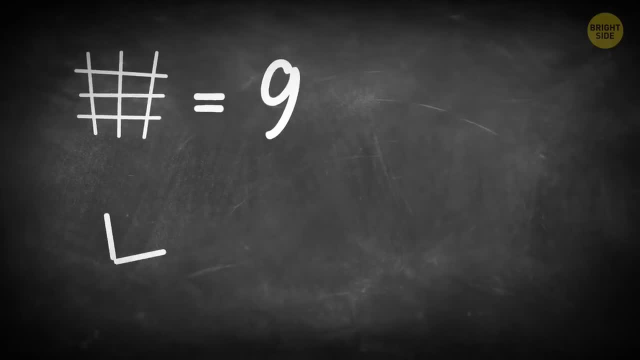 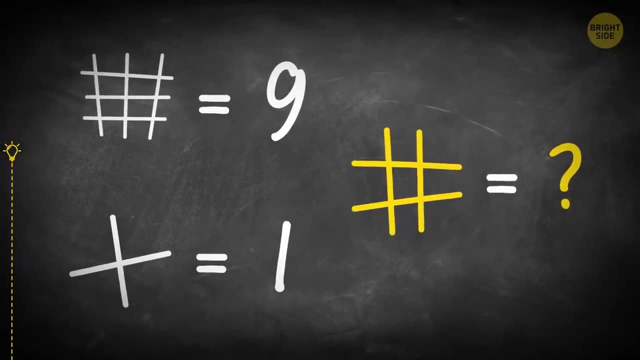 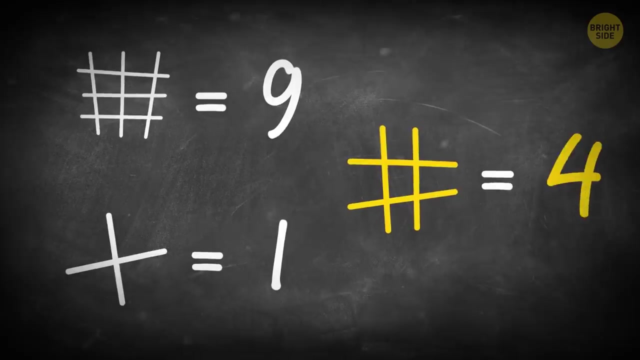 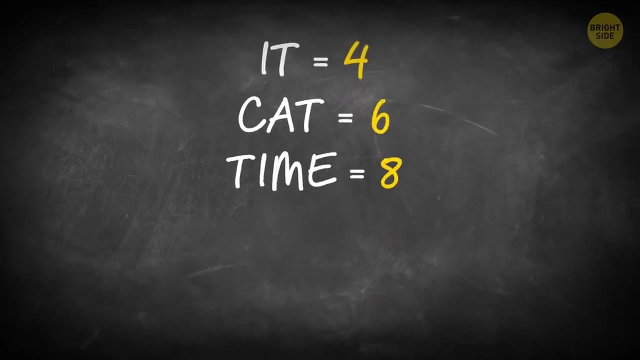 Look at the picture attentively and try to figure out which number should be there instead of the question mark. It should be 4.. That's the number of intersections. And how fast will you find the answer to this riddle? It equals 4.. Cat equals 6.. Time equals 8.. Hippo equals 10.. Cheetah equals what? 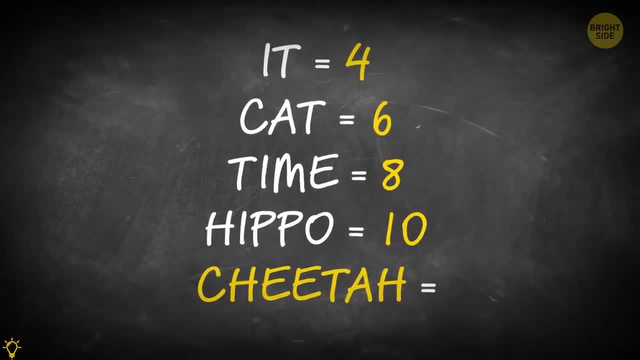 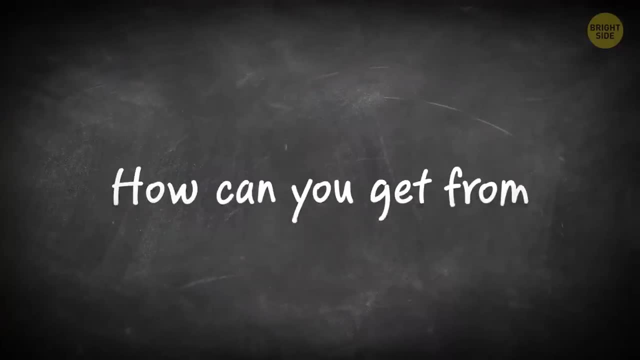 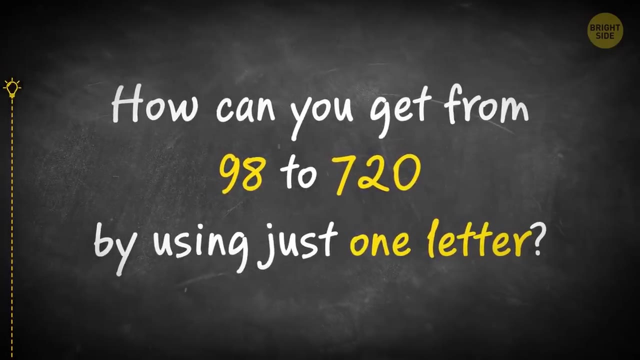 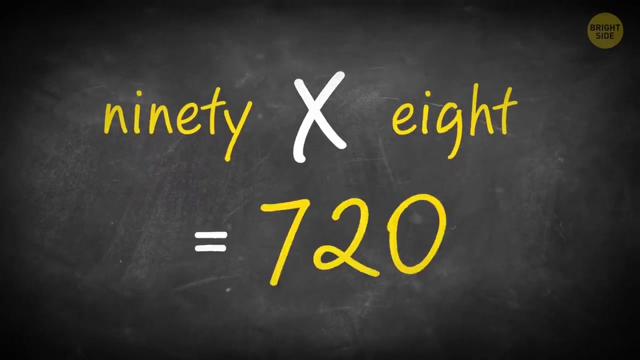 The correct answer is 14.. Each letter equals 2.. How can you get from 98 to 720 by using just one letter? Add the letter X between 90 and 8. You'll get 92.. Times 8 equals 720.. 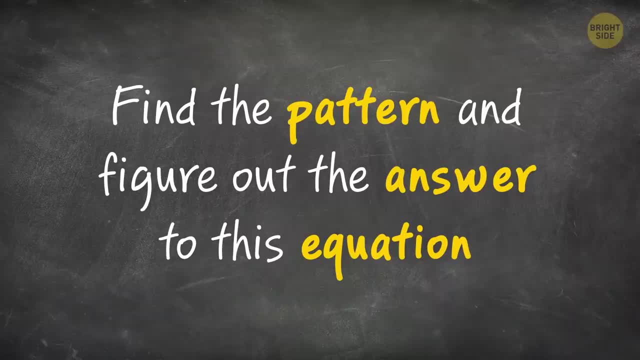 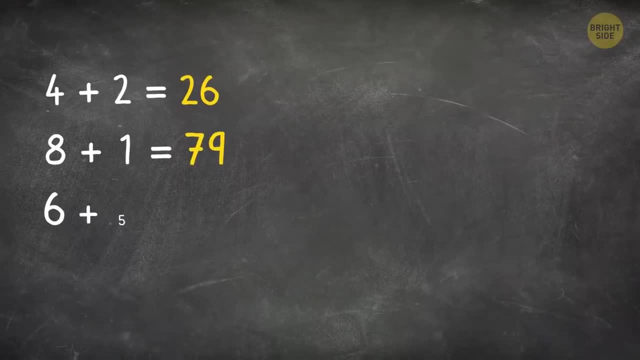 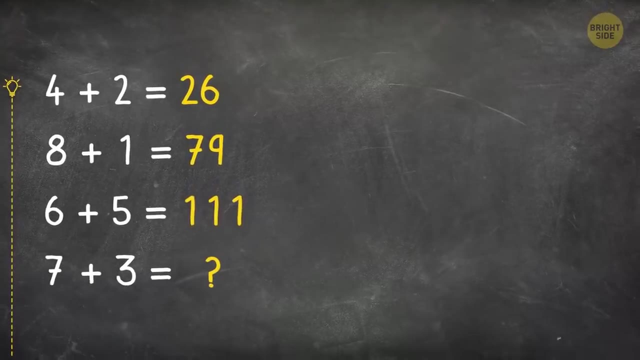 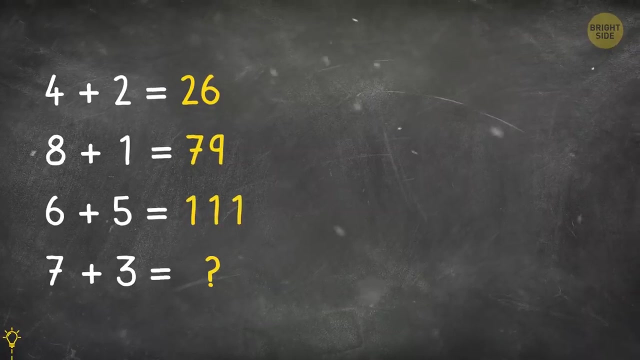 Can you find the pattern and figure out the answer to this equation? 4 plus 2 equals 26.. 8 plus 1 equals 79.. 6 plus 5 equals 111.. 7 plus 3 equals. 4 plus 2 equals 7.. 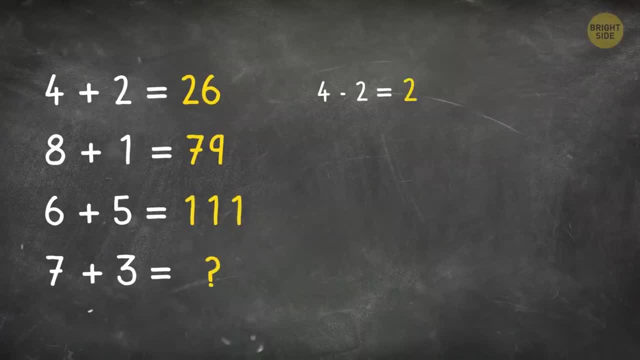 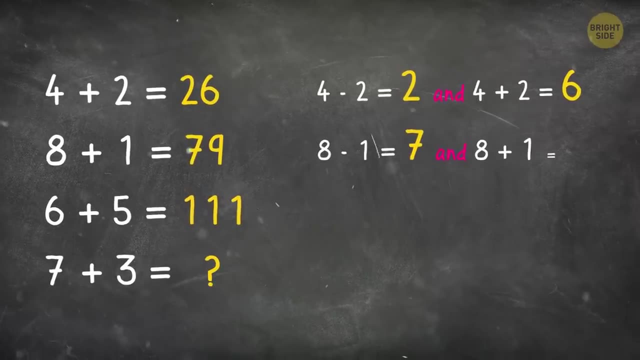 4 plus 2 equals 7.. 8 plus 1 equals 26,, since 4 minus 2 equals 2, and 4 plus 2 equals 6.. 8 minus 1 is 7, and 8 plus 1 equals 9, and so on. 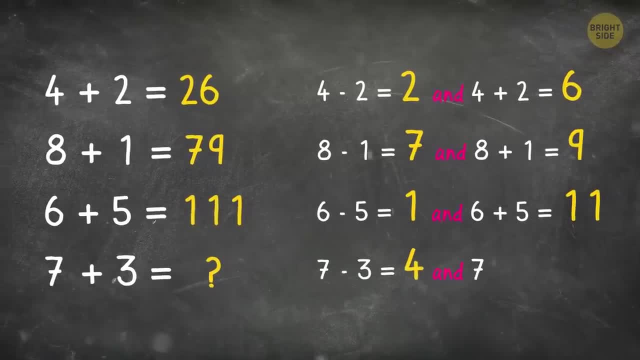 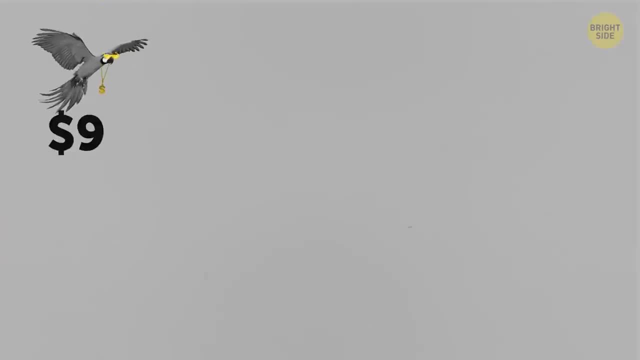 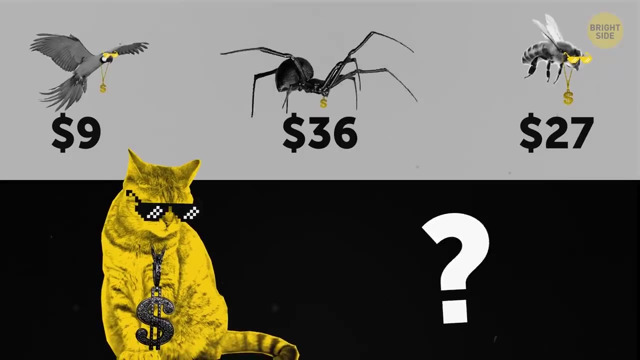 7 minus 3 equals 4, and 7 plus 3 equals 10.. It means the answer will be 410.. A parrot got $9,, a spider received $36, and a bee $27.. How much money will a cat get? 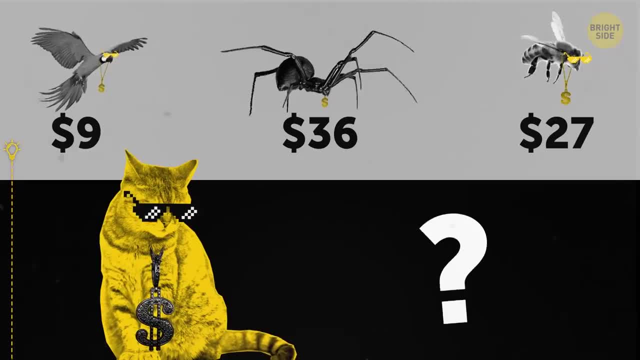 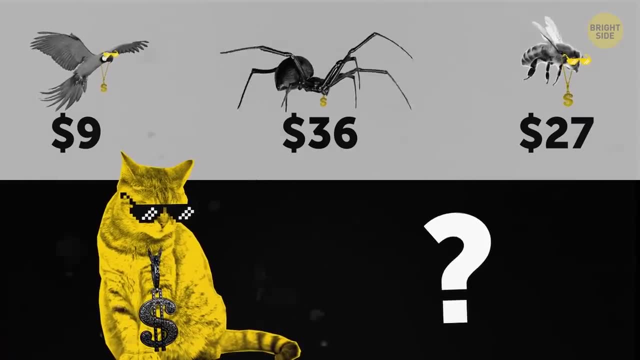 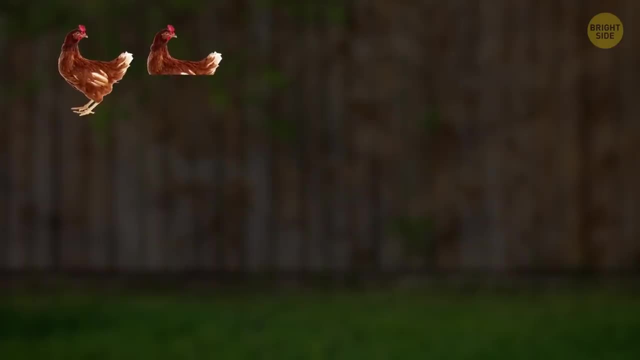 How many eggs will a half-a-dozen hens lay in a half-a-dozen days? Meow: 18 bucks, $4.50 for each leg. A hen and a half lay an egg and a half in a day and a half. 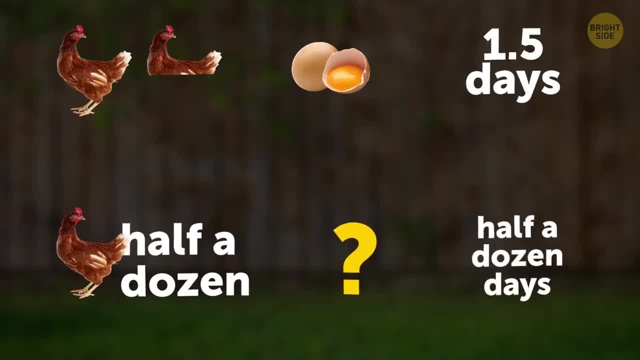 How many eggs will a half-a-dozen hens lay in a half-a-dozen days? How many eggs will a half-a-dozen hens lay in a half-a-dozen days? How many eggs will a half-a-dozen hens lay in a half-a-dozen days? 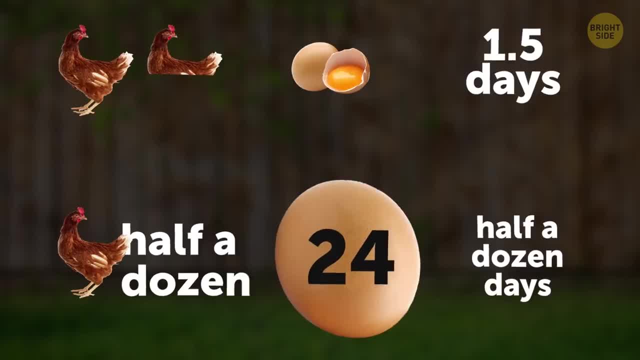 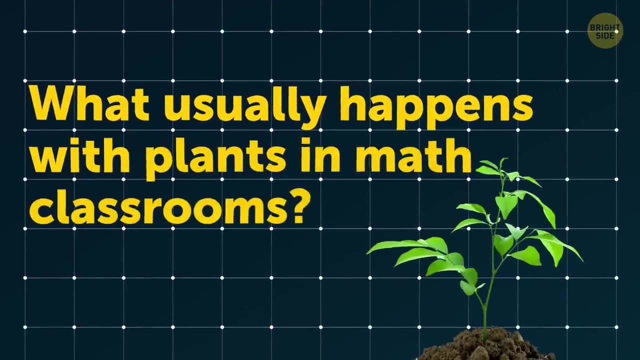 24.. If there are 4 times more hens and they have 4 times more days, they will lay 16 times more eggs. 16 times 1 and a half equals 24 eggs. Now what usually happens with plants in math classrooms? 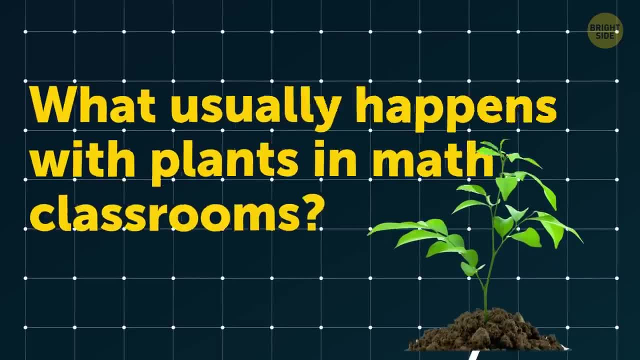 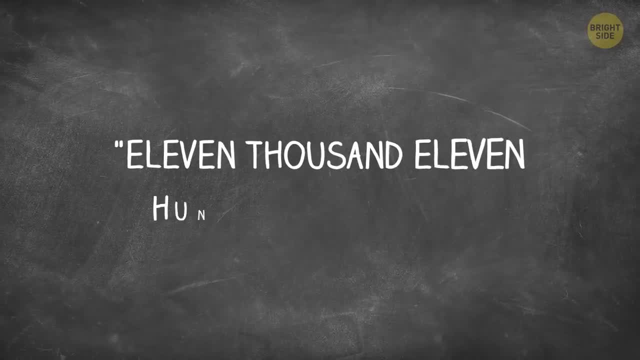 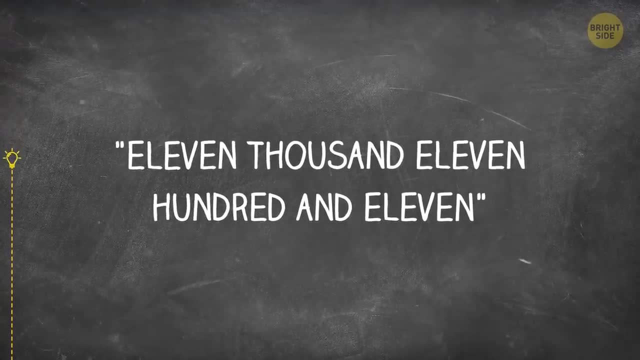 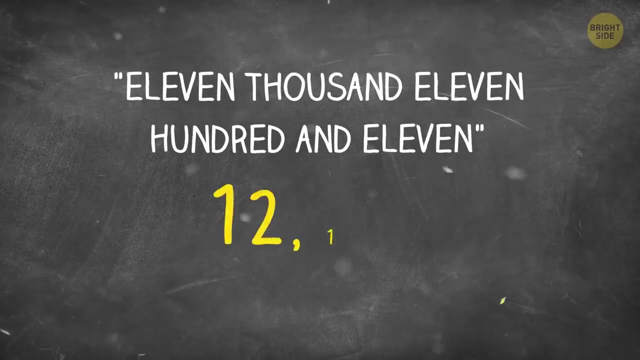 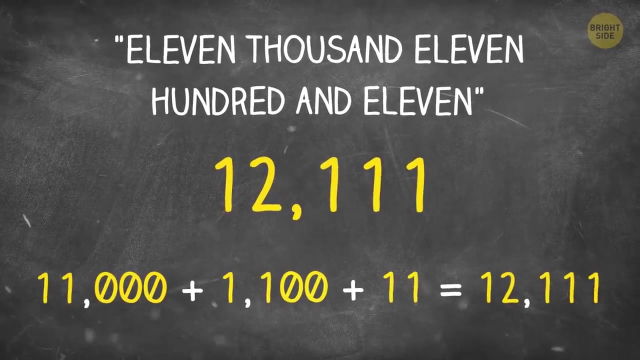 They grow square roots. How can you write 11,000, 1100, and 11 in digits? It'll be 1-2-1-1-1.. 11,000 plus 1100 plus 11. Equals 12,111.. 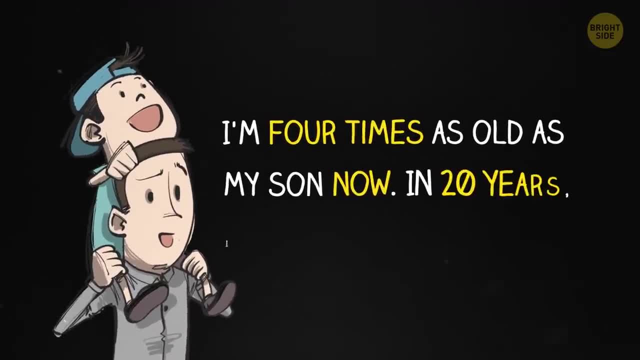 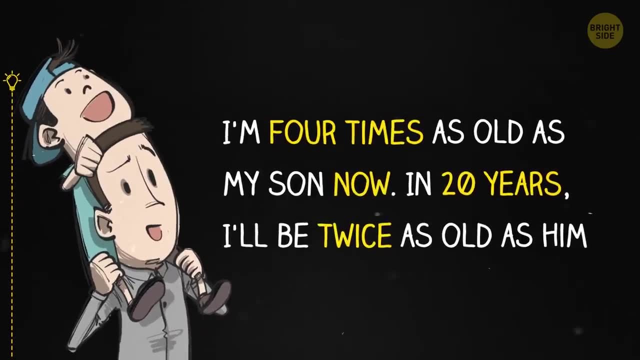 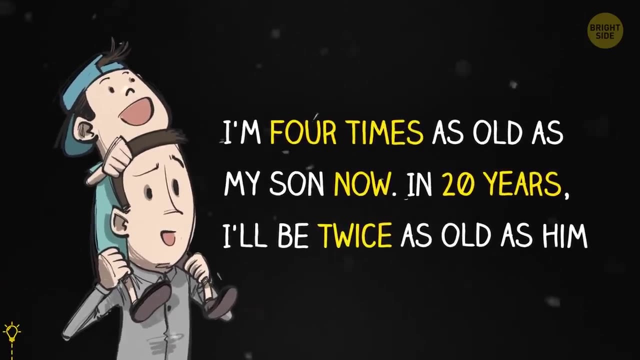 Now I'm 4 times as old as my son now. In 20 years, I'll be twice as old as him. How old are we now? I'm 40, and my son is 10.. I'm 40, and my son is 10.. 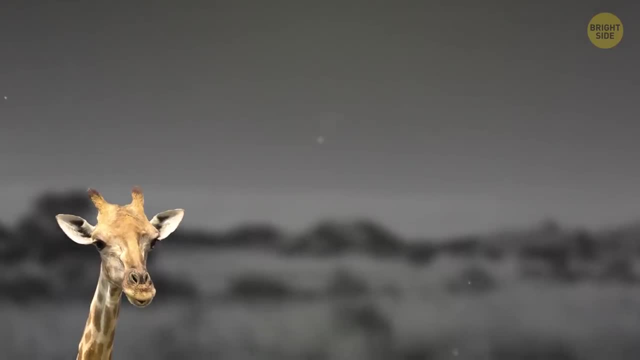 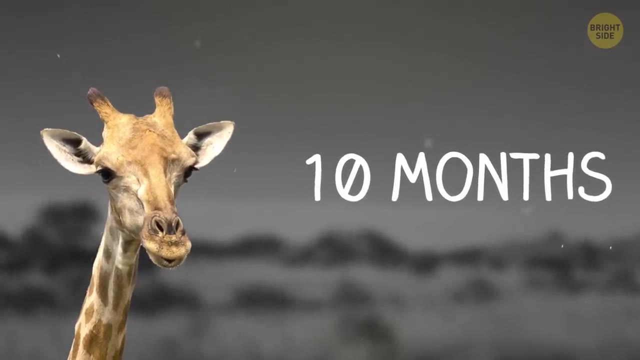 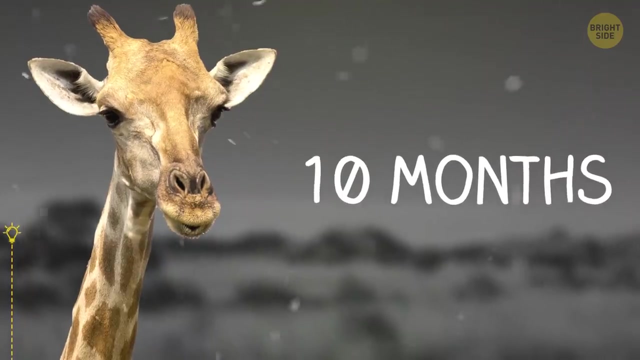 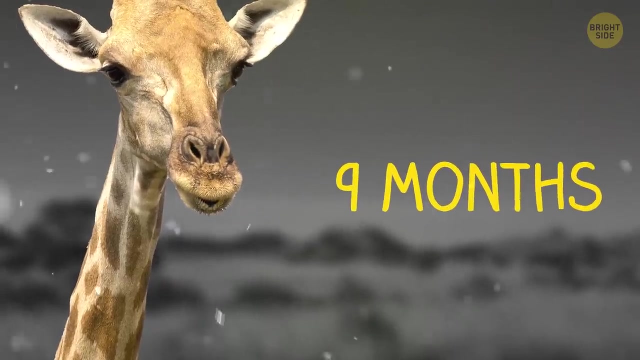 A baby giraffe doubled in height Every month until it reached its dad's size. It took 10 months. How many months did it take the baby giraffe to grow half its current size? 9 months, Because the animal doubled in height every next month. 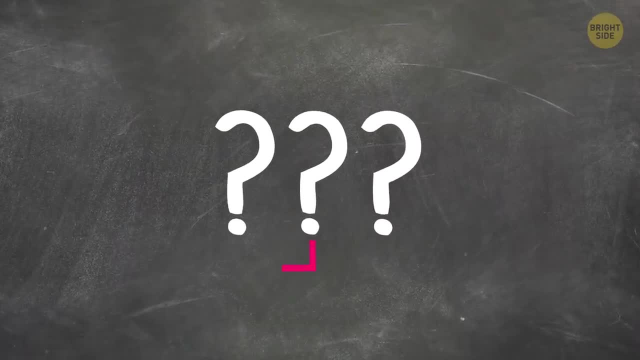 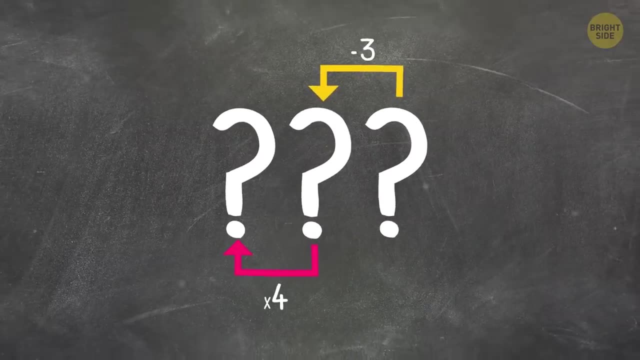 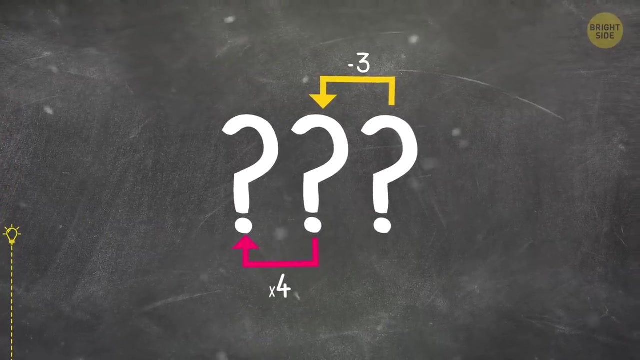 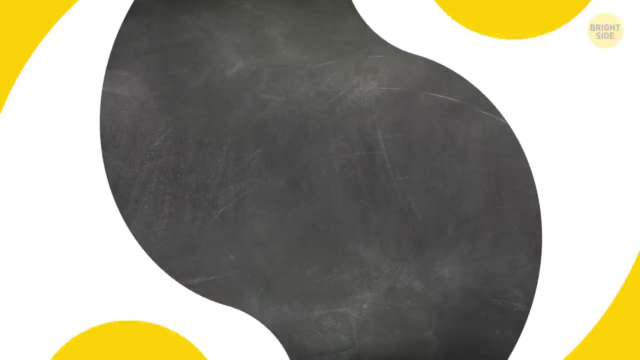 I'm a 3-digit number. My second digit is 4 times as big as the first one And the third digit is 3 less than the second. What number am I? I'm 141.. The whole positive numbers have a 2-digit answer when added. 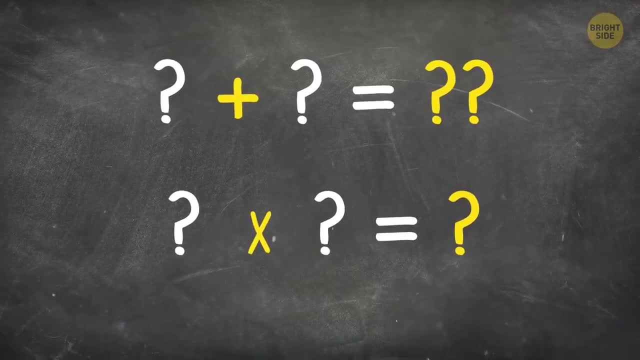 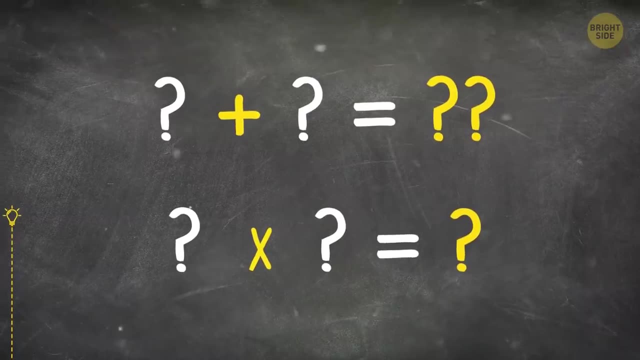 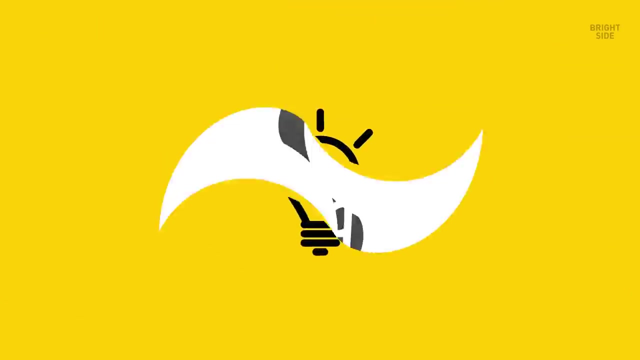 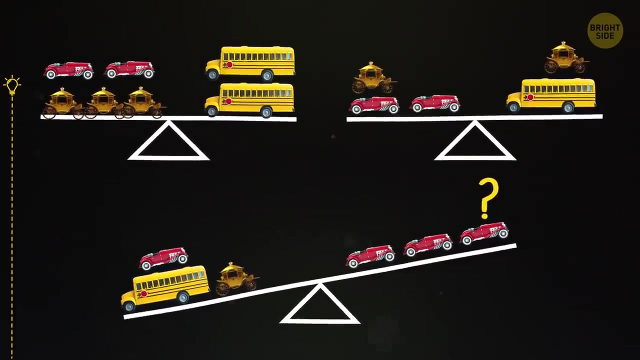 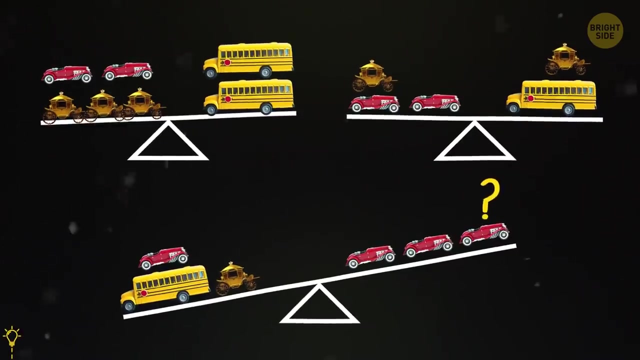 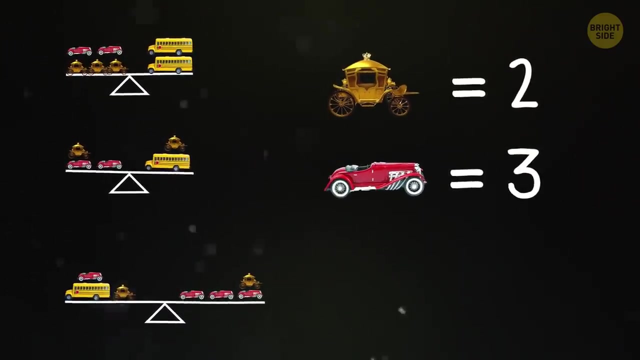 and a 1-digit answer. when multiplied, What are these numbers? They're 1 and 9.. Which vehicle do you need to add to make the scale balance? A carriage. A carriage equals 2,, a car equals 3, and a bus equals 6.. 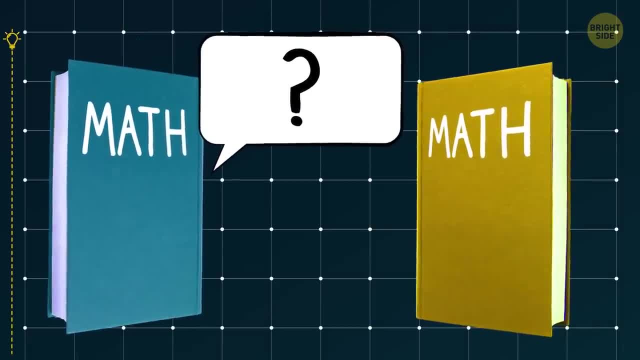 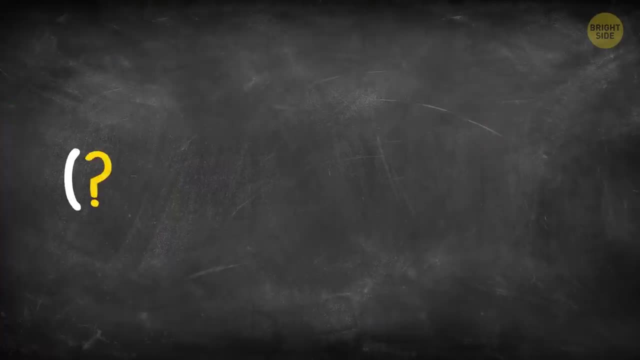 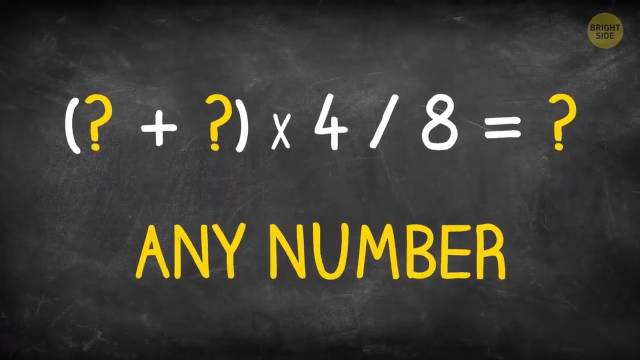 What did one math book tell another? I have so many problems. Add me to myself and multiply by 4.. Then divide me by 8, and you'll have me once again. What number am I? I can be any number. Try it out. 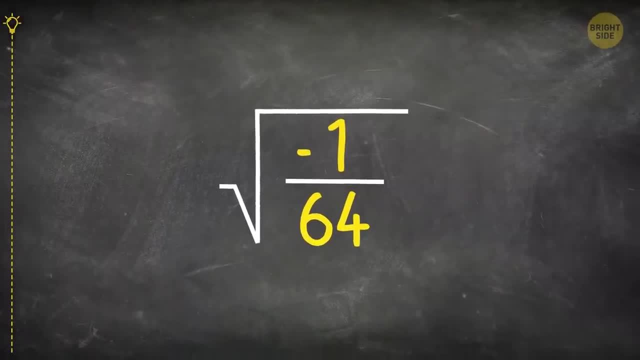 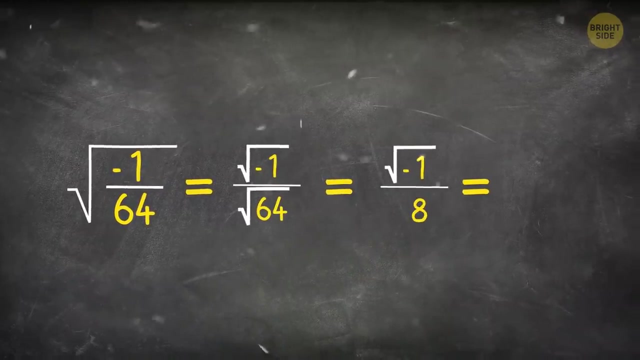 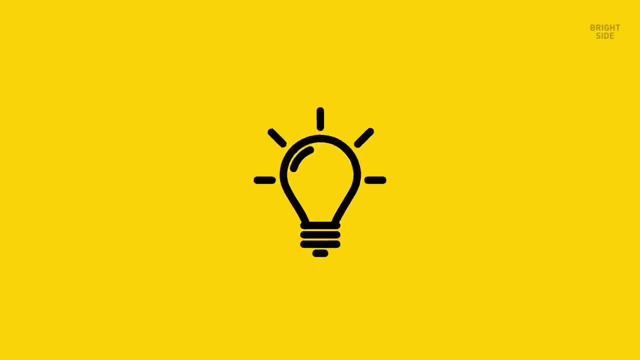 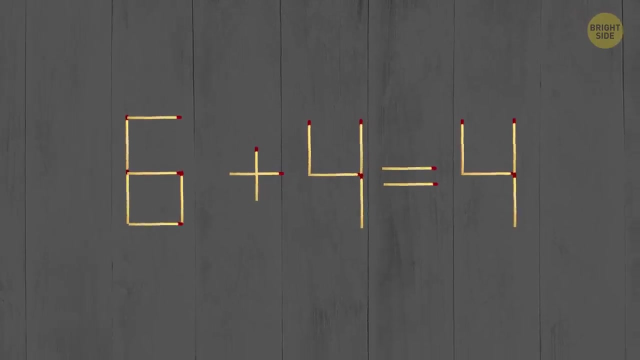 Can you guess what this rebus means? The answer is: I over 8.. You have an equation made of matchsticks: 6 plus 4 equals 4.. Move just one matchstick. to make it true, You'll need to take one matchstick. 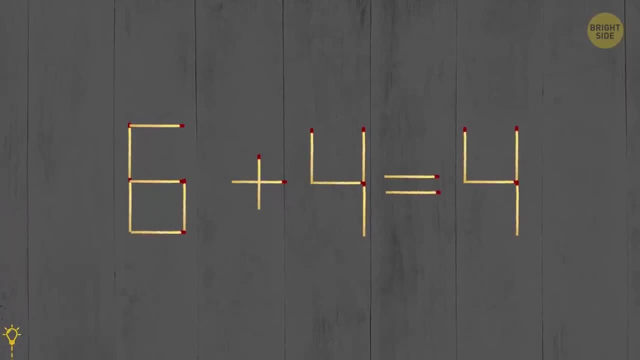 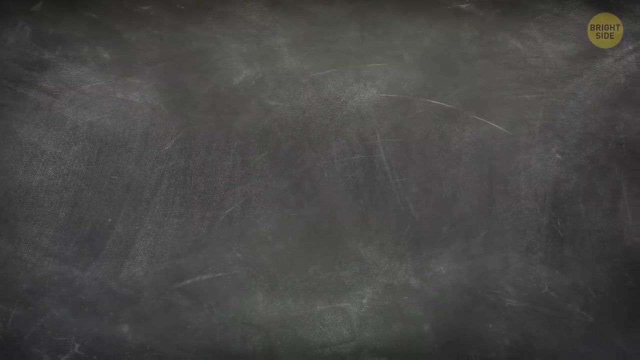 You'll need to take one matchstick from the plus sign and add it to 6 so that it makes 8.. Then you'll have 8 minus 4 equals 4.. I'll give you three clues and your task is to find a 4-digit number. 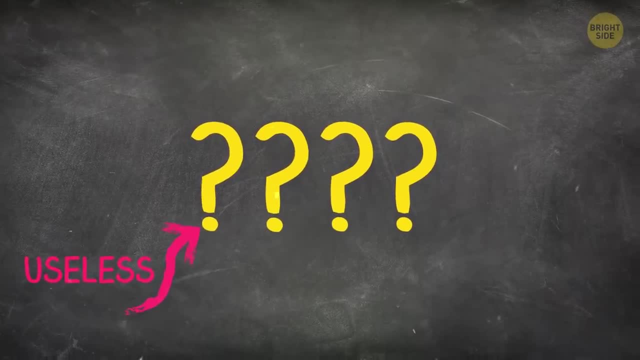 Its first digit is useless. The second and fourth digits are the mirror images of each other, And the third digit is half the same. The third digit is half the same, The third digit is half the same And the fourth digit is half the same. 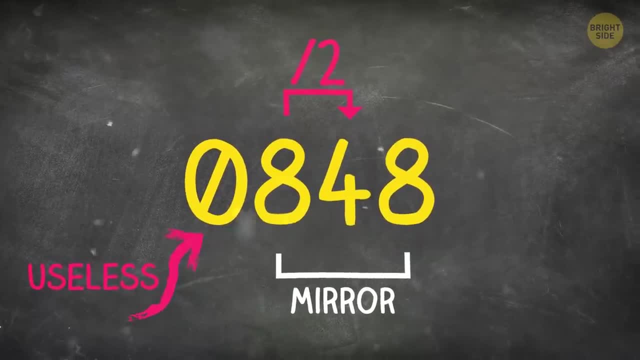 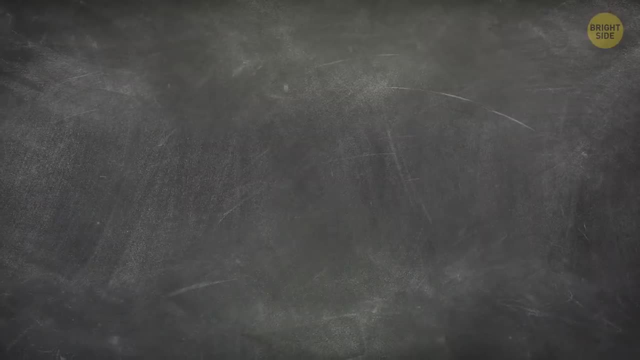 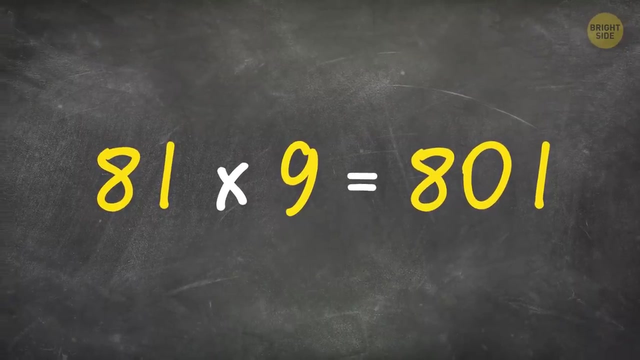 This number is 0-8-4-8.. 0 is the number of no use, 8 mirrors each other and 4 is half of 8.. Look at this equation: 81 times 9 equals 801.. What can you do to make this equation correct? 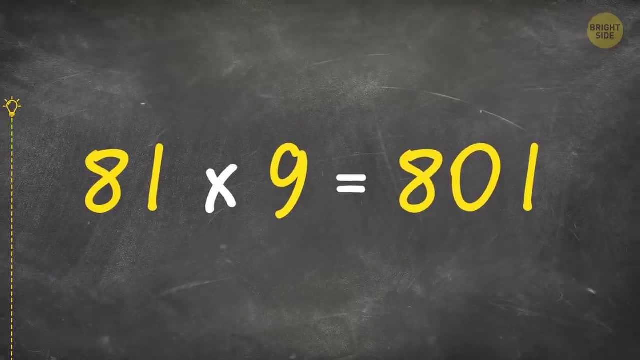 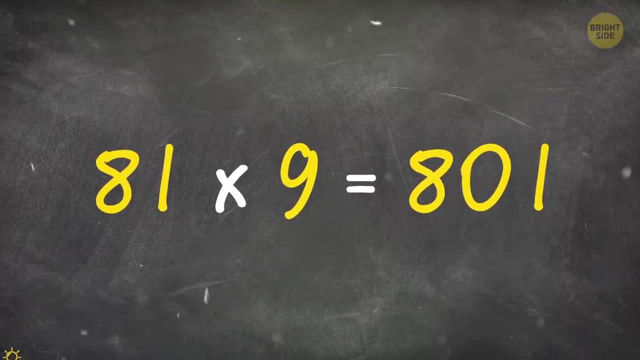 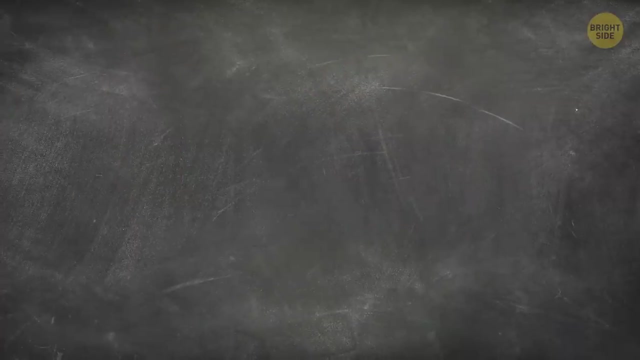 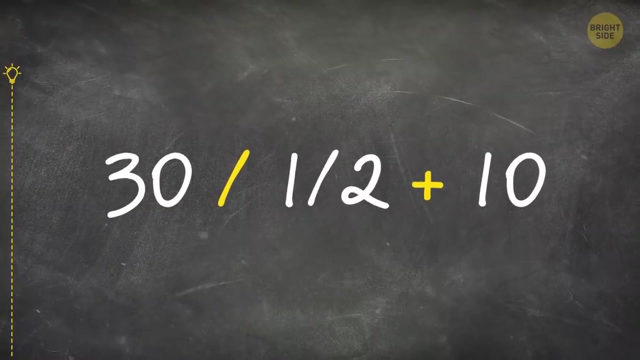 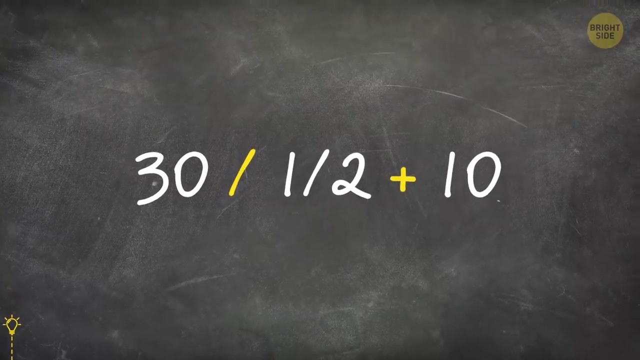 Look at this equation, Turn it upside down: 108 equals 6 times 18.. Divide 30 by 1 half and add 10.. What will be the result? What will be the result? It's 70. Most people count like this. 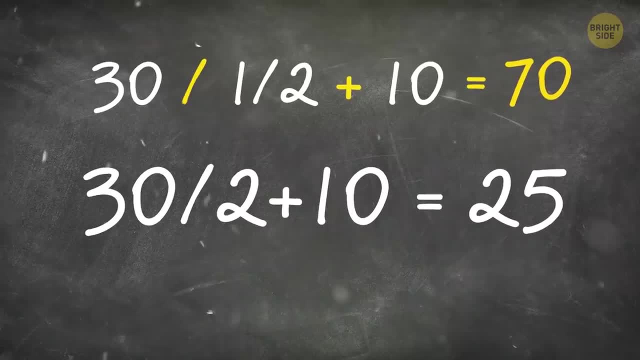 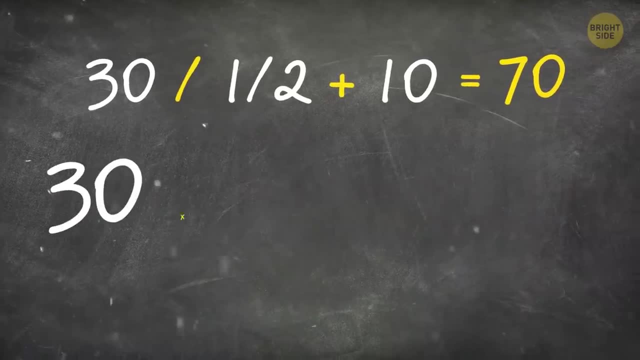 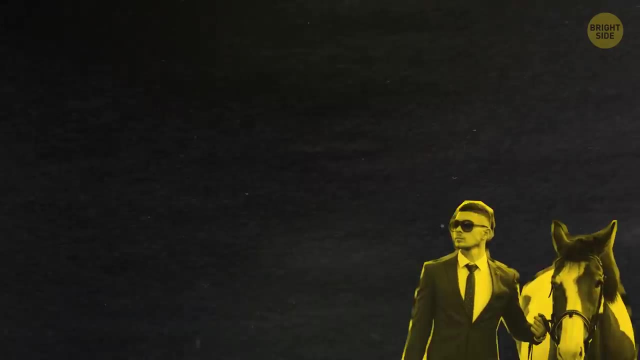 30 divided by 2 plus 10 equals 25. But when you divide some number by fraction, You actually have to multiply it by the inverted fraction. So 30 times 2 plus 10 equals 70. Horses and people are gathered in a stable. 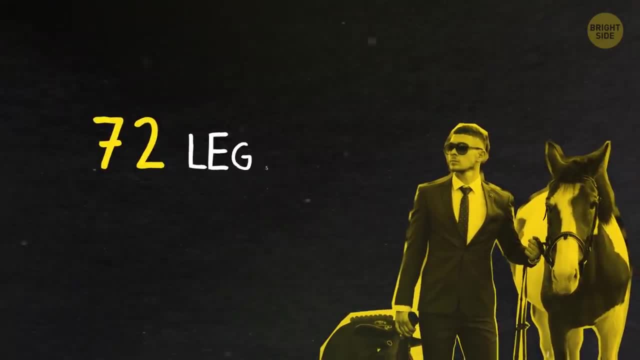 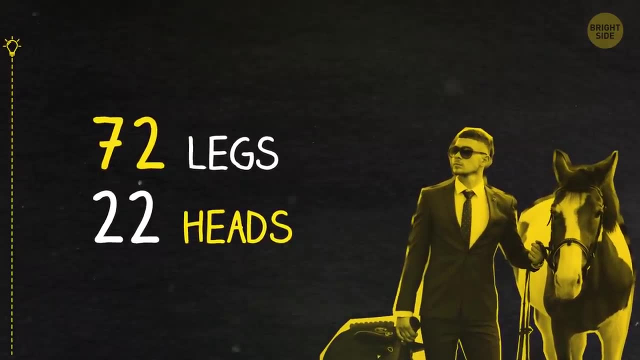 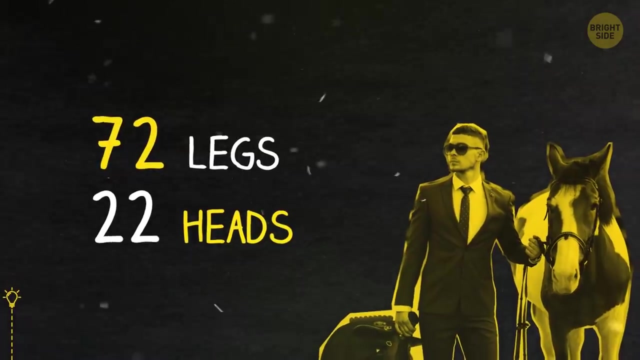 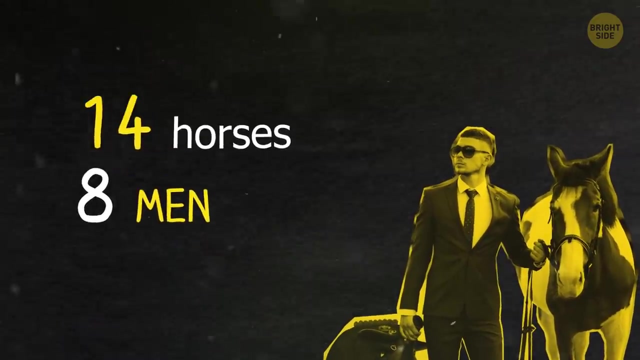 You know that in total, There are 72 legs and 22 heads. How many horses and how many people are there in the stable? There are 14 horses and 8 men. 14 plus 8 equals 22 heads. 14 plus 8 equals 22 heads. 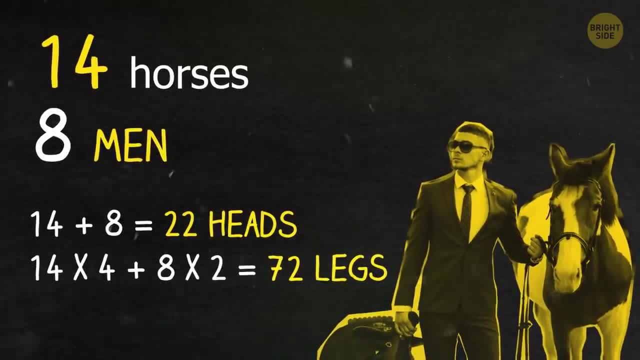 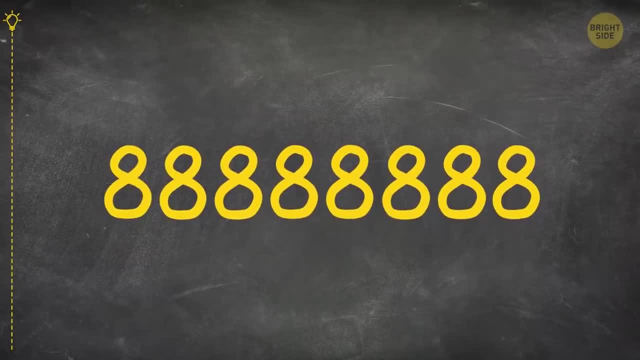 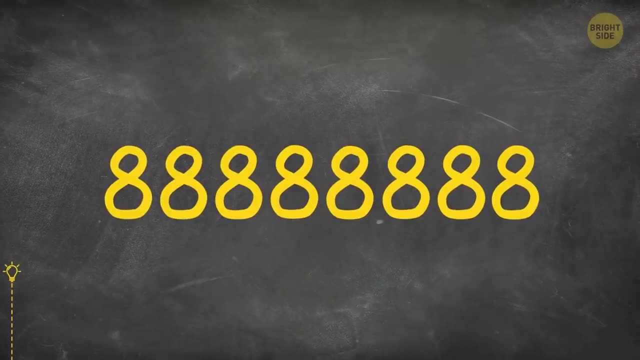 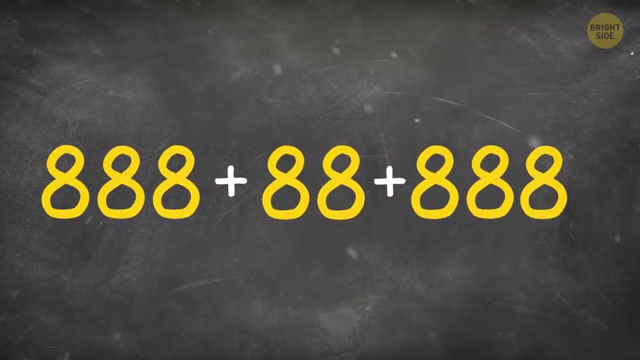 14 times 4 and 8 times 2 equals 72 legs. Write down 8 eighths so that they add up to 1,000. 888 plus 88 plus 8 plus 8 plus 8 equals 1,000. 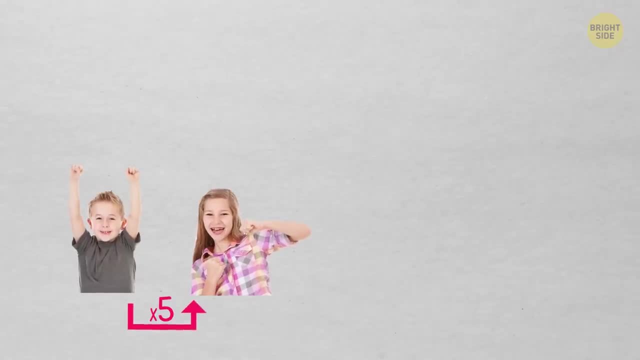 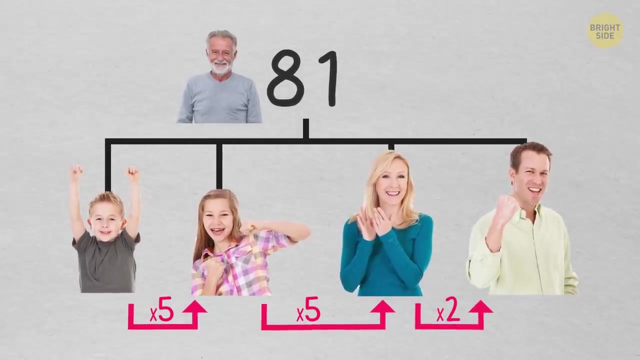 My daughter is 5 times as old as my son. My wife is 5 times as old as my daughter. I'm twice as old as my wife, And my grandfather, who celebrated his 81st birthday yesterday, Is as old as all of us together. How old is my daughter? 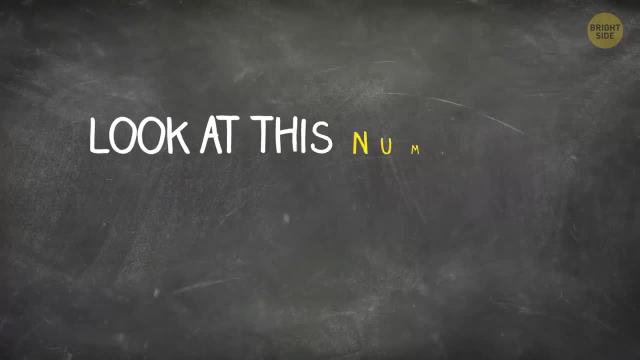 She's 5 times as old as my son. She's 5 times as old as my daughter. She's 5 times as old as my son. She's 5 times as old as my son. Look at this numerical series And figure out its logic And the next number. 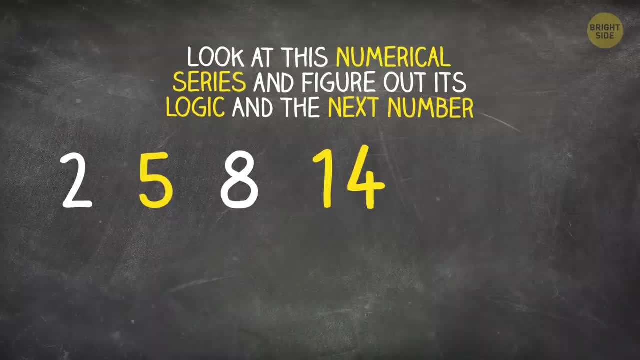 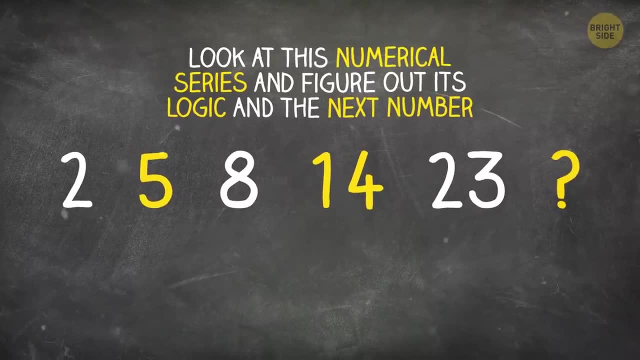 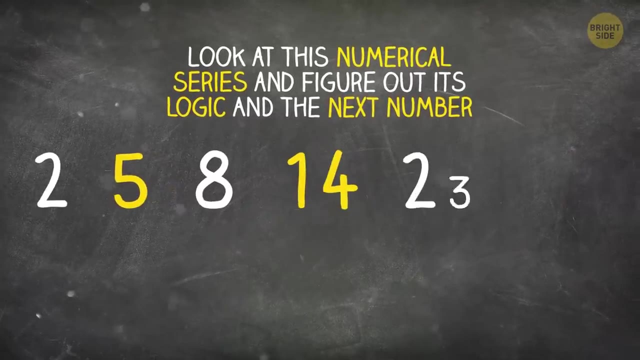 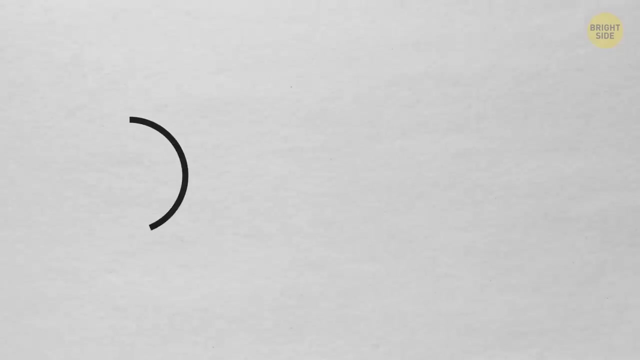 2,, 5,, 8,, 14,, 23, The next number will be 38. Every time you increase the sum of the previous numbers by 1, The next number will be 38. A circle has two, a point has zero and a sphere has three. 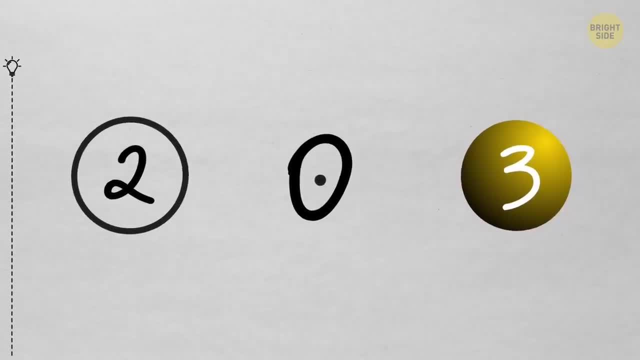 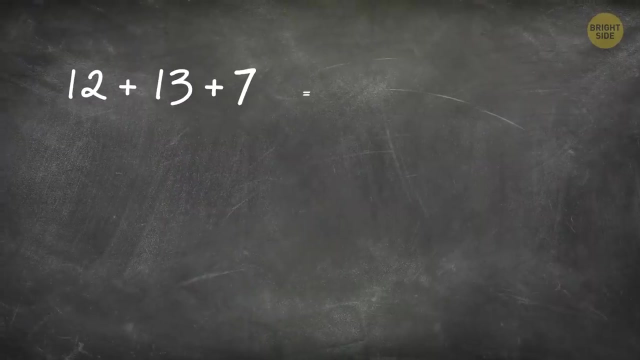 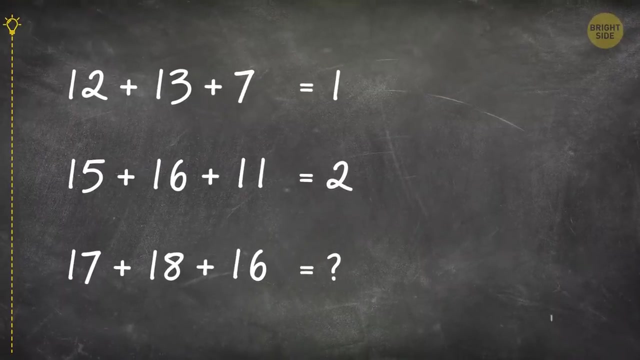 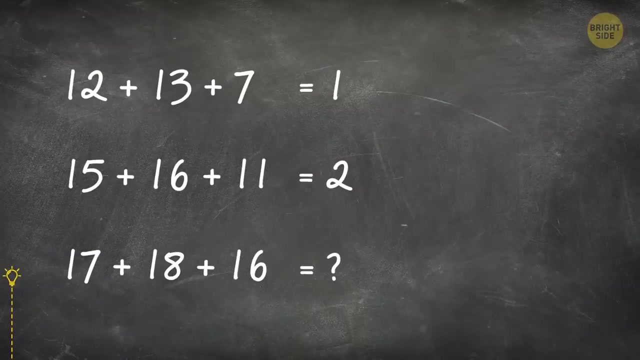 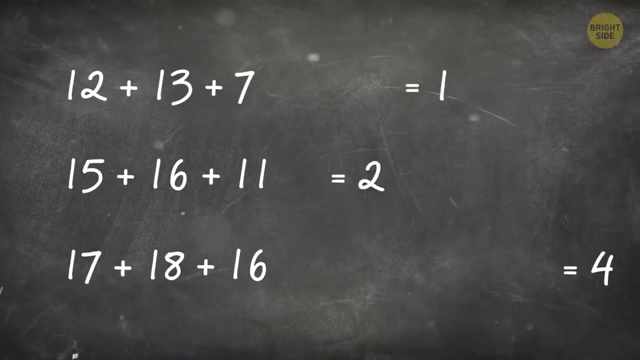 What am I talking about? Dimensions? Try to understand the logic used in the following question and figure out what number can replace the question mark. The correct answer is 4.. 12 plus 13 plus 7 equals 32.. 3 minus 2 equals 1.. 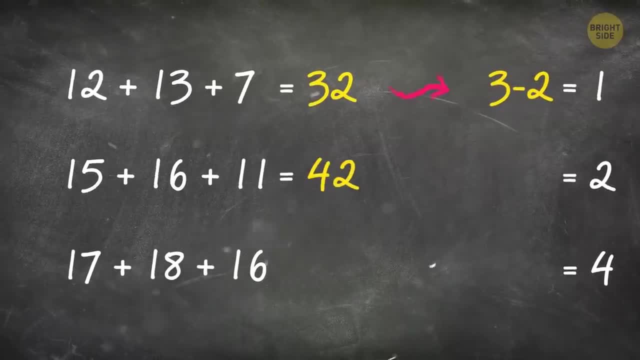 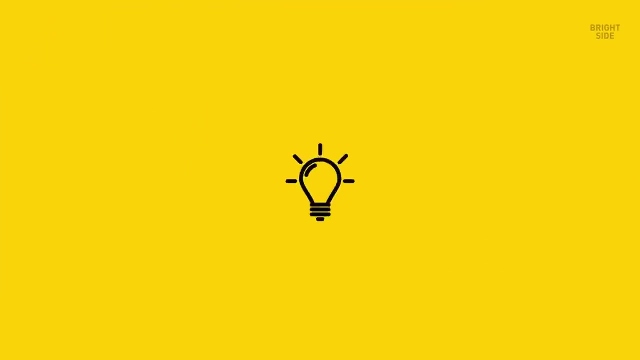 15 plus 16 plus 11 equals 42.. 4 minus 2 equals 2.. 17 plus 18 plus 16 equals 51. So 5 minus 1 equals 4.. How can you take 2 from 5 so that it leaves 4?? 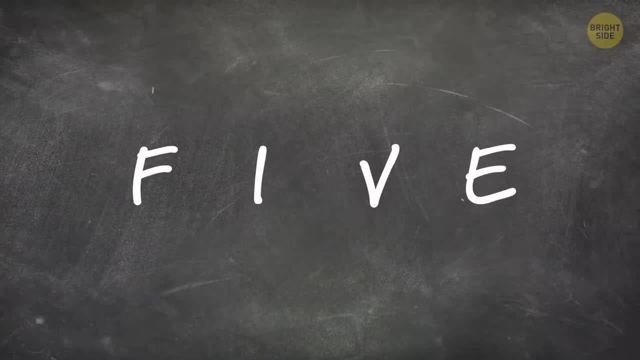 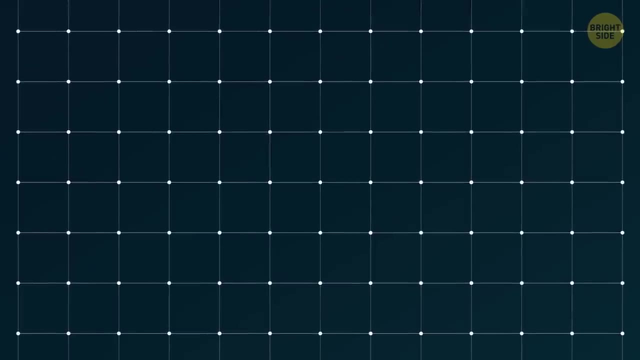 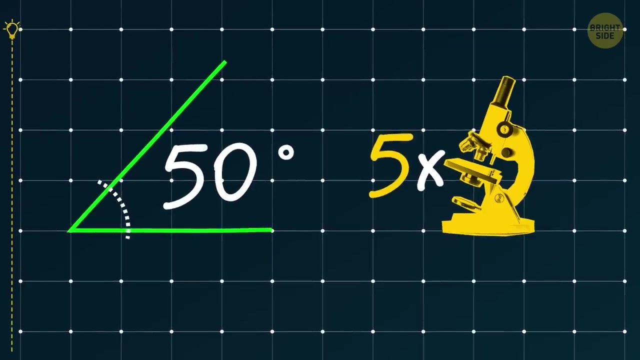 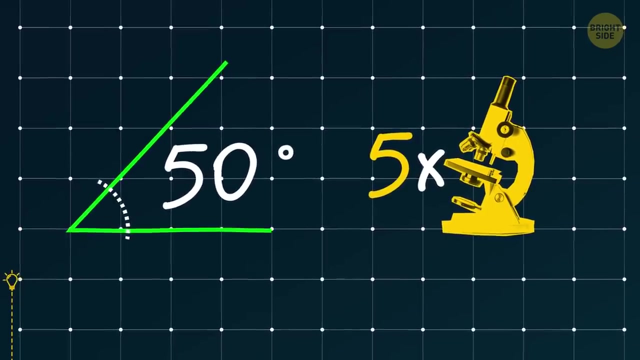 Write down the word 5 first, Now remove the F and E and you get the Roman numeral IV. How much will a 50-degree angle measure if you look at it through a microscope that magnifies 5 times? The angle won't change. 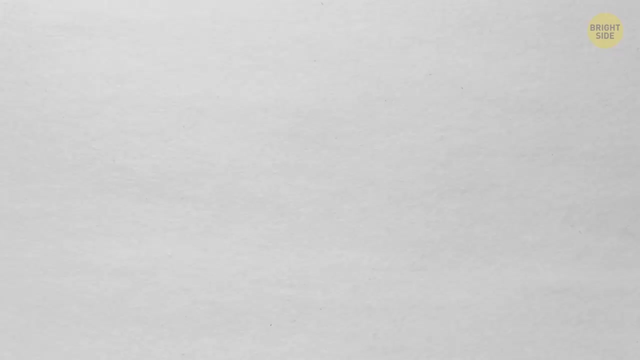 It'll still be 50 degrees. 1 is to 3, as 3 is to 5, and 5 is to 4.. Can you figure out the pattern? The word 1 has 3 letters, the word 3 has 5, and the word 5 consists of 4 letters. 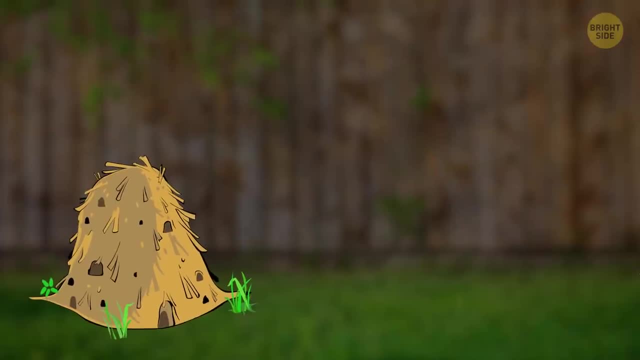 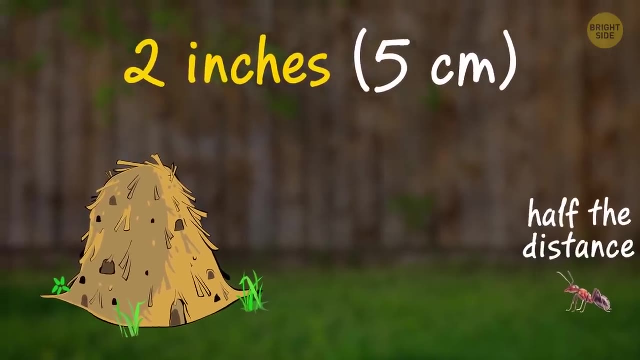 How many letters does an ant have? An ant is 2 inches away from its home. With every next step it covers half the distance to its home, But the door isn't always as deep, so I will just skip the first object. 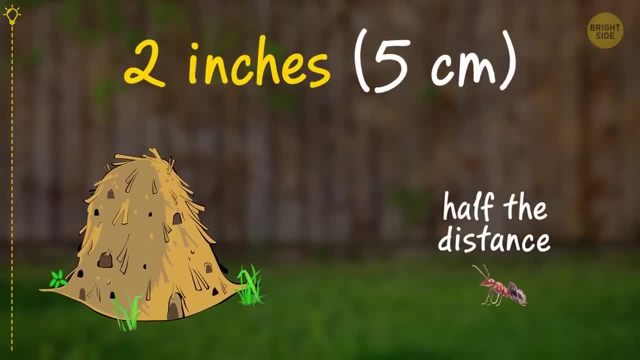 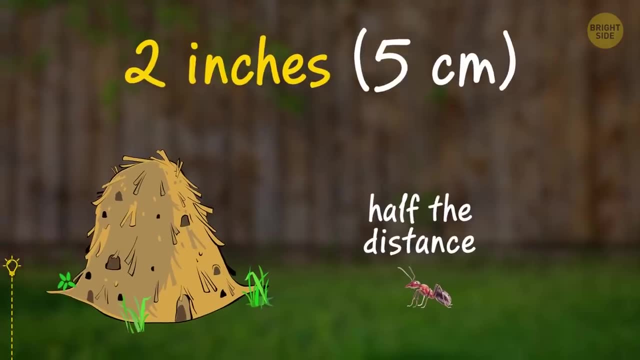 Also note the distance to the entrance. How many steps will it take the insect to reach its destination? 1, 6 steps. scary- 9 students. 30 students. 37 students. 38 students. 36 students. 4. break stairs. 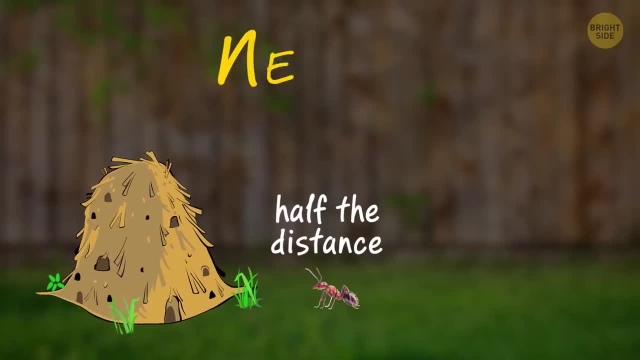 5. There is 4 walkway. The ant will never reach the door because every time it'll travel only half the distance. When you break the disappeared door, you break the bear's toes in the other way, and now try to crack the toughest one. 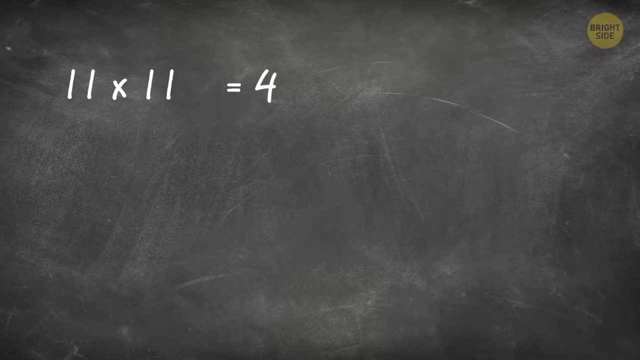 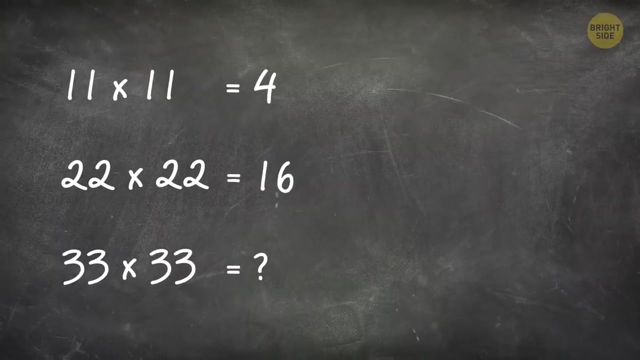 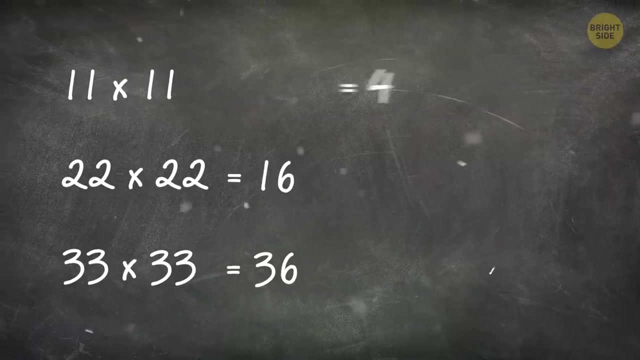 3 steps. scary 3 steps. serious. 11 times 11 equals 4,. 22 times 22 equals 8,. 13 times 2, 22 equals 16.. 33 times 33 equals 1.. The correct answer is 36.. 11 times 11 turns into 1 plus 1 times 1 plus. 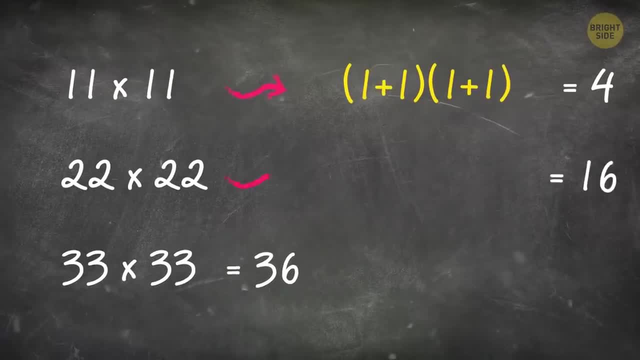 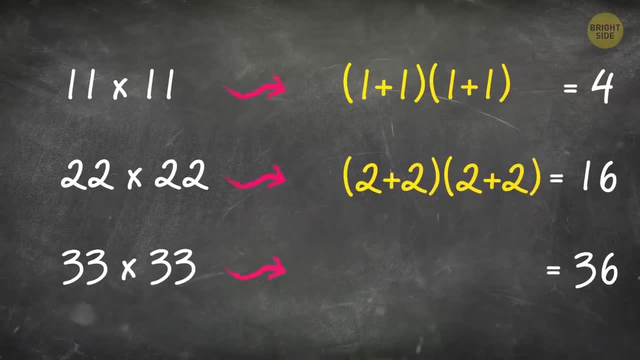 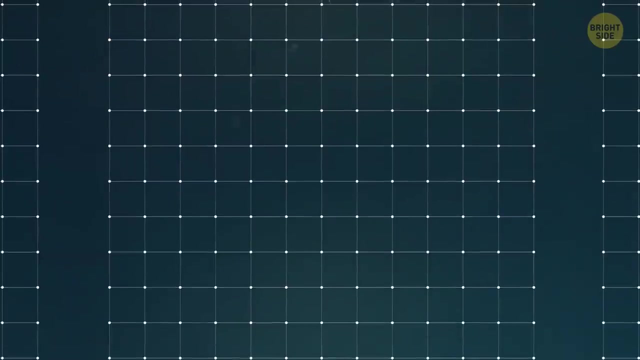 1 equals 4.. 22 times 22 turns into 2 plus 2. times 2 plus 2 equals 16.. 33 times 33 turns into 3 plus 3. times 3 plus 3 equals 36.. So let's see how good your math skills are. 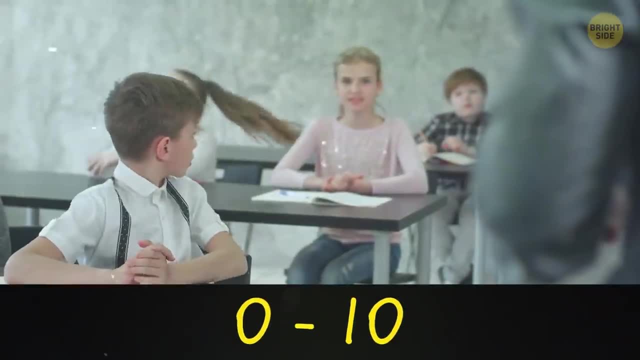 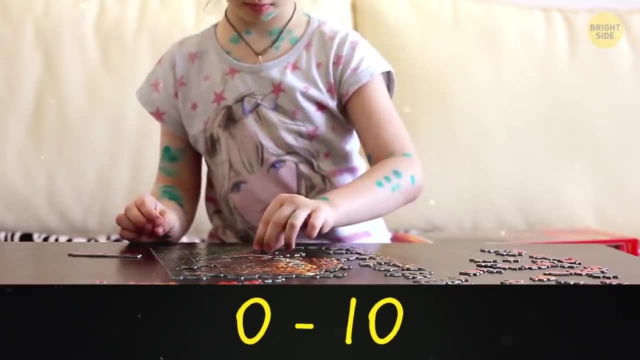 If you solved 0 to 10 riddles, you probably didn't pay much attention to math at school. Start with the easiest puzzles and try to crack at least one a day. Soon you'll see the results. Do you have 11 to 24 correct answers? Not. 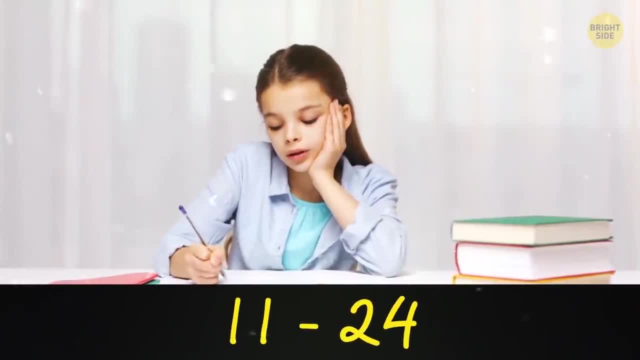 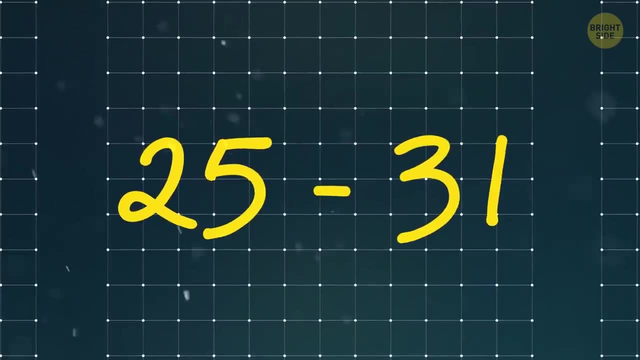 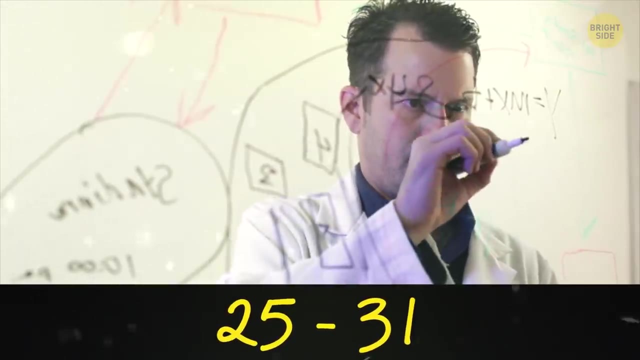 bad. You're likely to use math now and then in your everyday life. Do you know what can make you even better? Yeah, practice. If your score is 25 to 31, solved riddles, congrats. You must be some math genius. But don't stop practicing or your skills will. 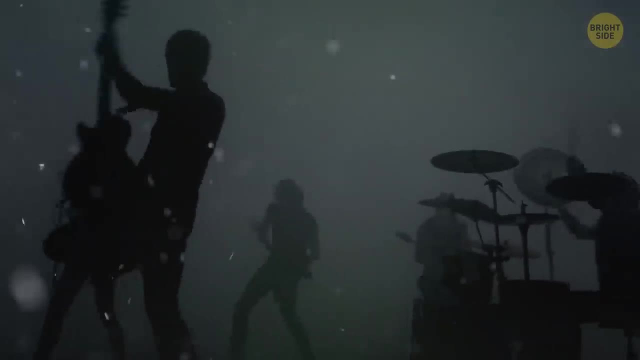 get rusty. Like Jack Black said in School of Rock, get off your a** and do some math. Subtitles by the Amaraorg community.